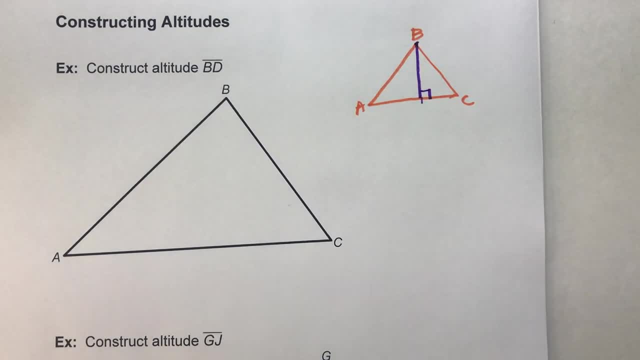 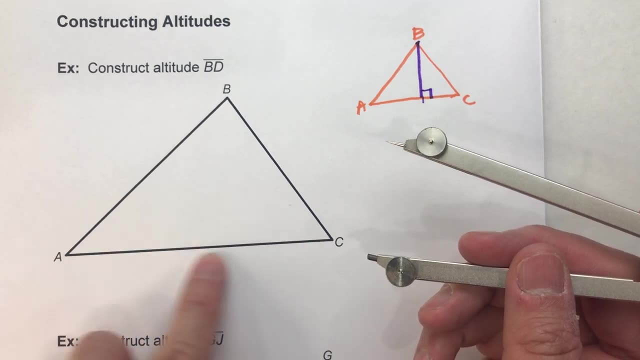 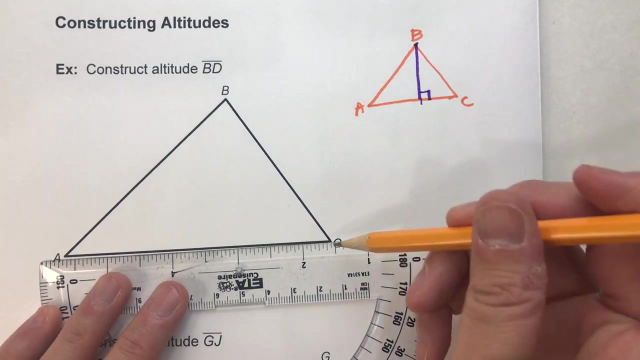 but goes through point B, just like that. Now, in order to construct that, we are going to basically construct the perpendicular to this through this point. Okay, now to do that. first thing I'm going to do is I'm going to extend this line, segment AC, a little bit in both directions. 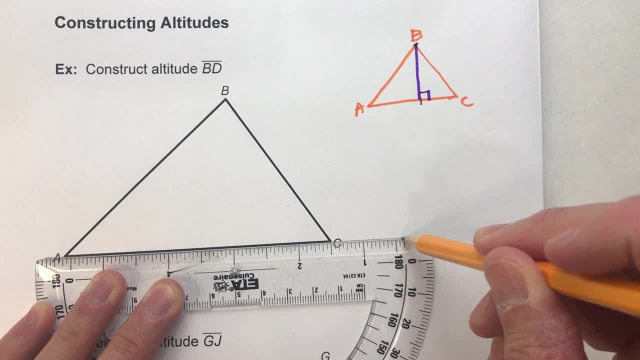 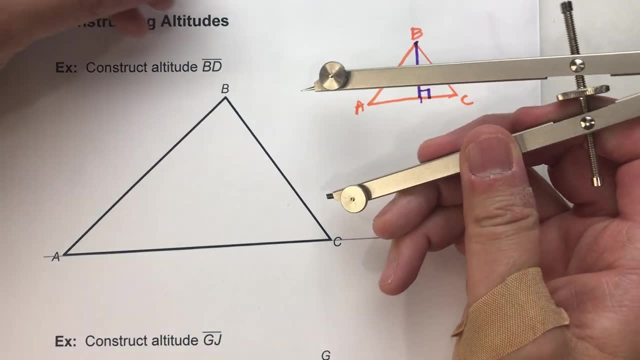 because we're going to need some length on this thing. So I'm just going to make it a little bit longer here, just in case we need it. Okay, you may or may not need it. Now I'm going to use my compass, setting from point B. 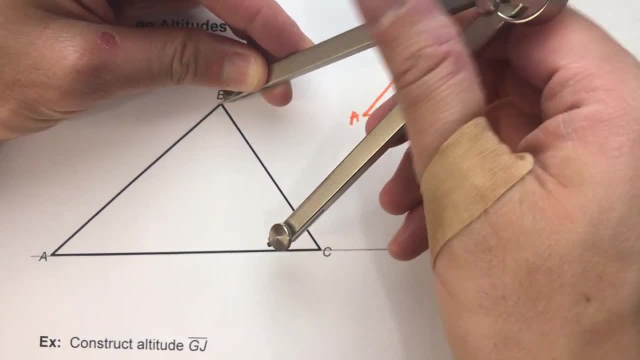 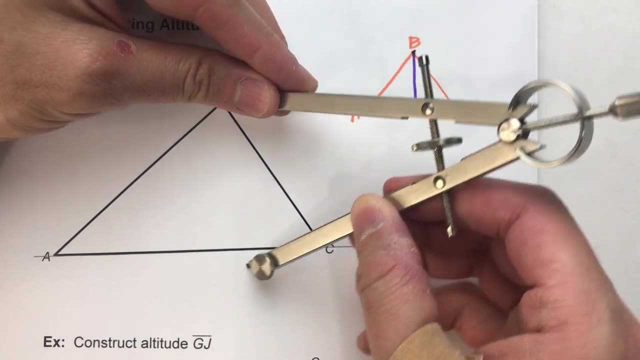 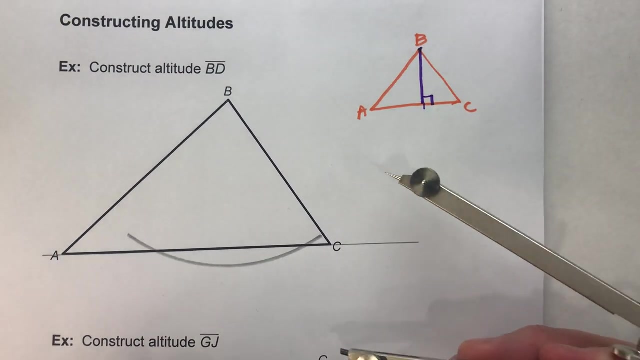 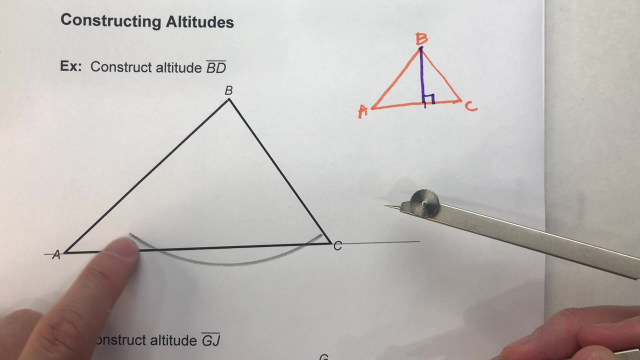 And I'm going to make it long enough so that it hits that line segment in two different places. Alright, so that looks pretty good, right? So I'm going to swing my arc and hit it in two spots. Alright, Now, from there, I'm going to go off each intersecting spot. So see where the arc. 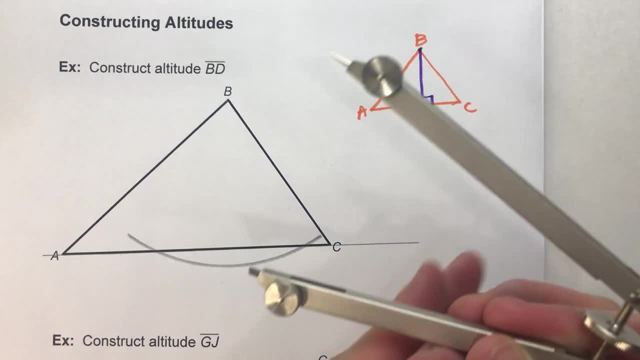 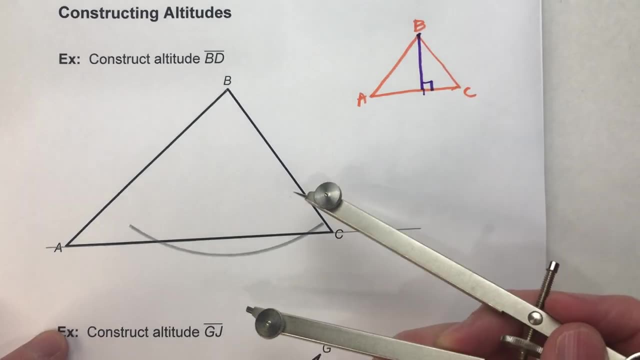 intersects the segment here and it intersects there. I'm going to take my compass setting and doesn't have to be the same as before. I'm going to make it a little smaller because I'm a little stronger room, But it does have to be more than half the distance from where the arc. 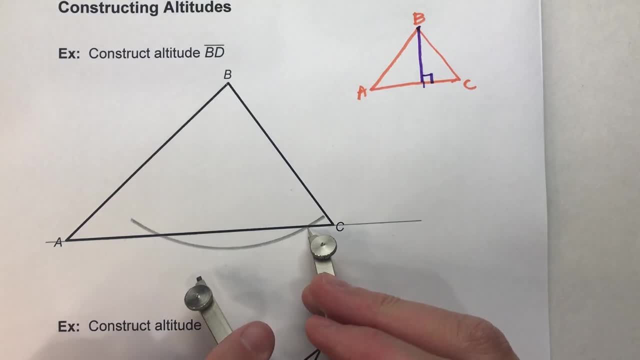 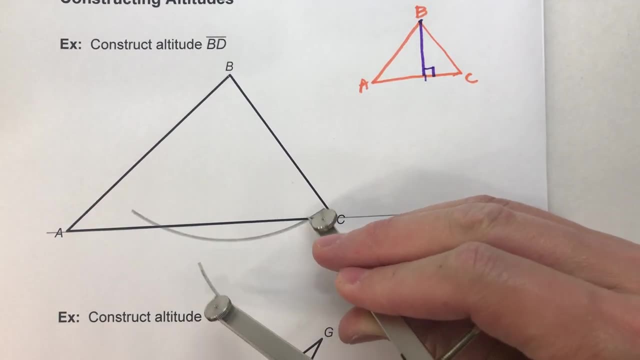 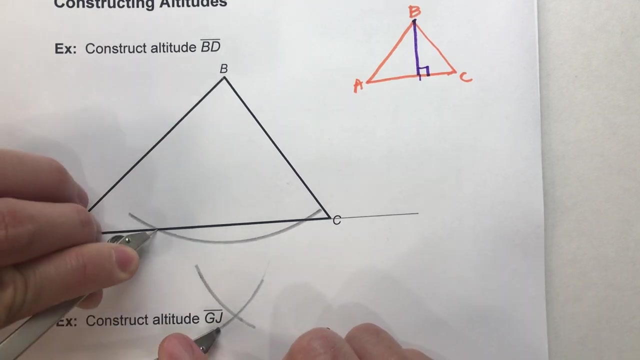 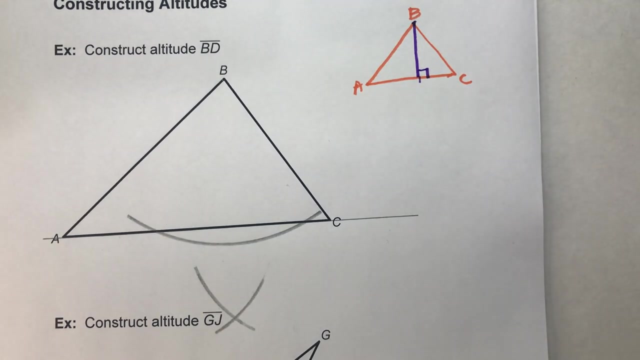 hits the line segment. Okay, But from here I'm going to take my compass and swing an arc down below on one side, And then, using that same compass, setting on the other side, and swing an arc. Now what am I basically doing? I'm basically doing the same construction that we've done. 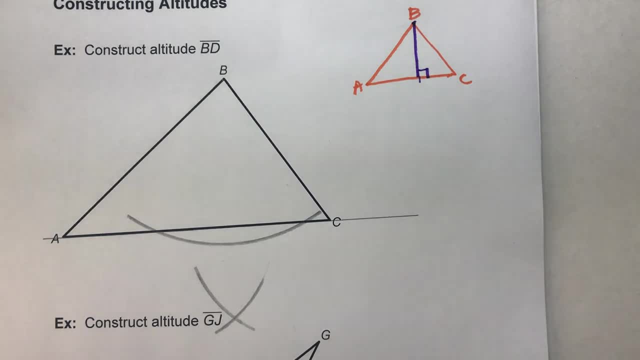 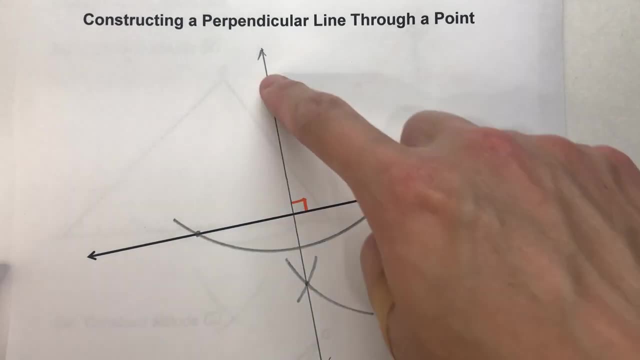 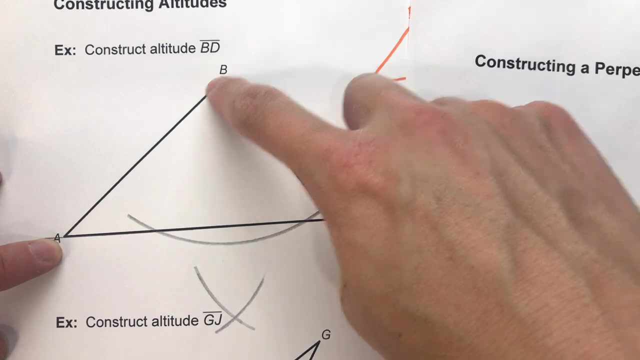 before. We've done this construction of constructing a perpendicular line through a point. When you have a line and a point and you're constructing a perpendicular through it, that's basically what we're doing Here. we have a line and we're we could almost ignore the rest. 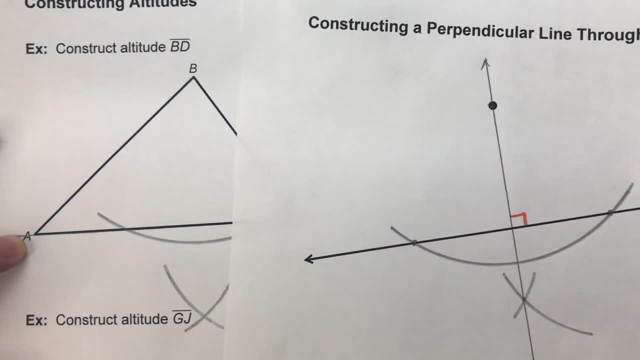 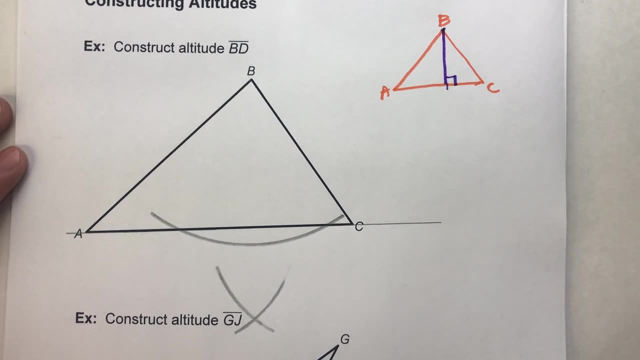 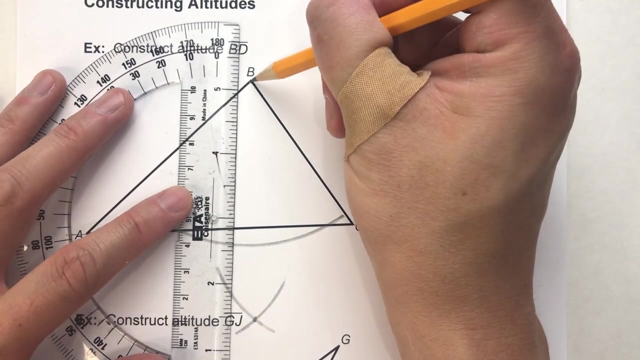 of the triangle and focus on that point B, And we're basically doing that exact same construction on this triangle. Okay, So I've got my point right here. then I'm going to draw my line through. So I'm going to go from B to that point, right there. 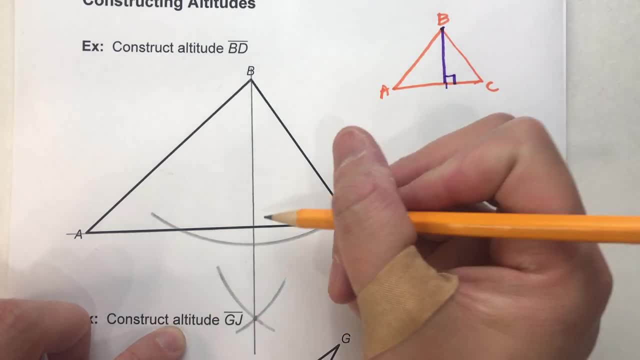 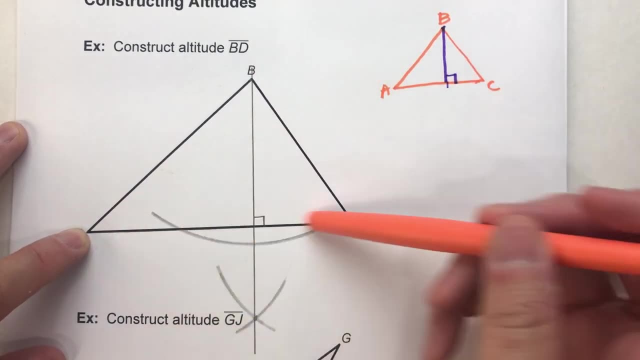 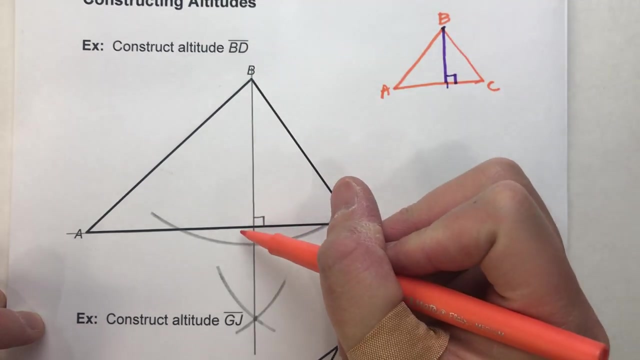 And I know this is perpendicular, because I basically constructed a perpendicular And that's all we really need for an altitude: a perpendicular through that point B. All right, we do need to name it. segment BD Here's B. So this will be D. this point right here will be D. 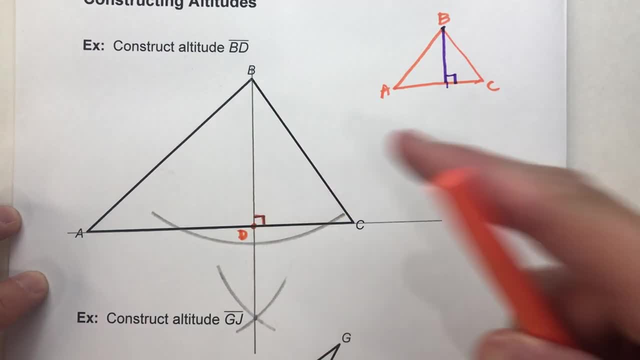 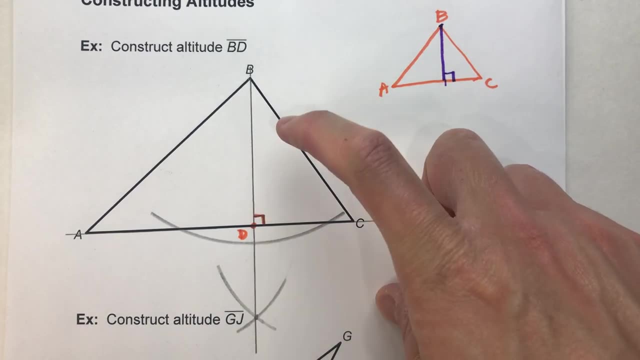 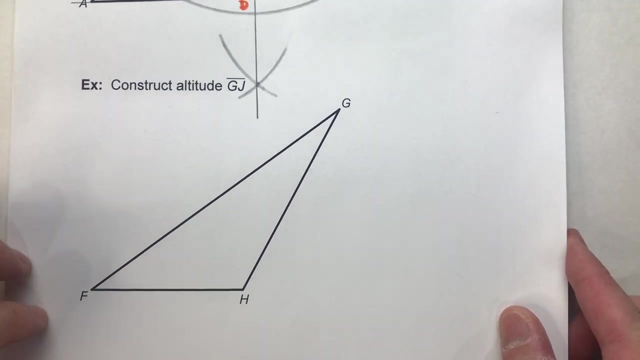 And we know it's perpendicular there, And this is my altitude. Okay, Now notice: this altitude is inside of the triangle. It's not always going to be inside the triangle, So that's why I have a second example for you. All right. this one says: construct altitude G. 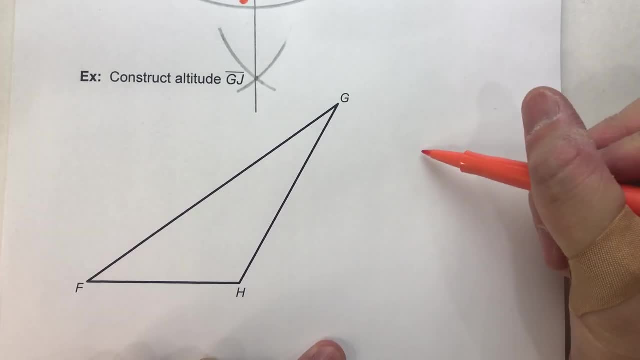 J. So again I'm going to do a little sketch so we can kind of picture what's going on here. So this time we have a triangle that kind of sticks out a bit. So here's G Okay And an altitude for. 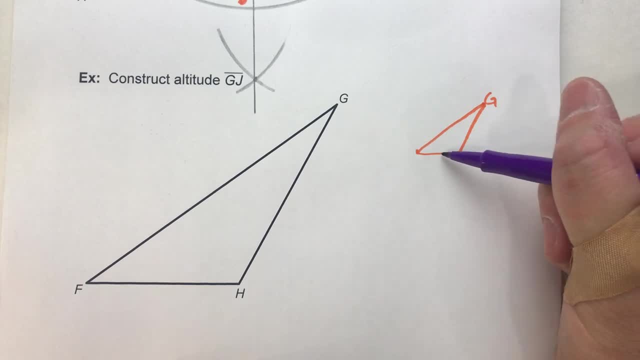 this would go from G perpendicular to the opposite side. But in order for it to be perpendicular to this opposite side, it's going to actually have to go down this way. And imagine this side being extended. it would be perpendicular like that And that's the construction we're going to have to do. 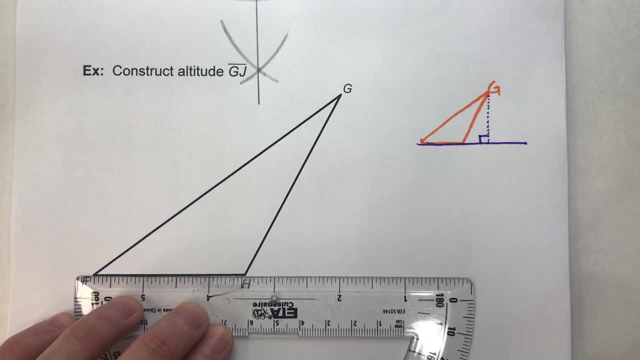 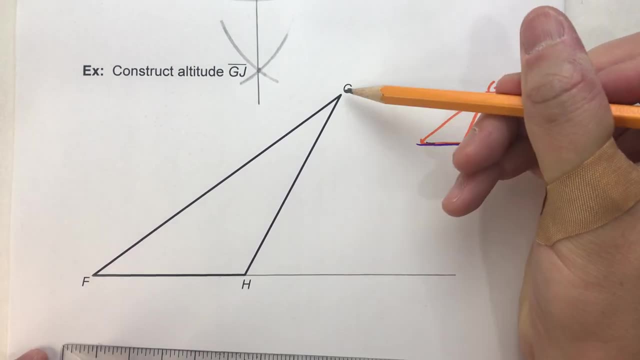 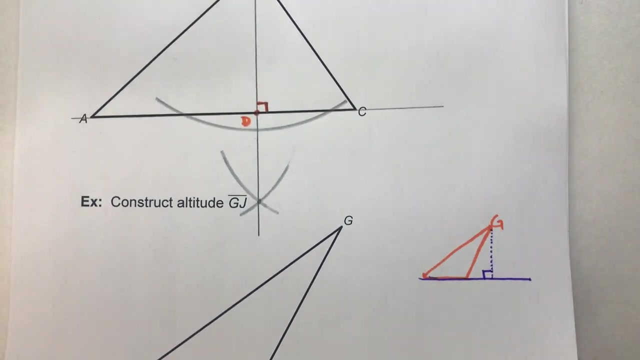 Okay. so the first thing we're going to do, I'm going to extend this side, because we're going to need this side to go further out. you can already kind of tell the altitude is going to be over here somewhere, All right, But once we've extended it out now, it's not much different than 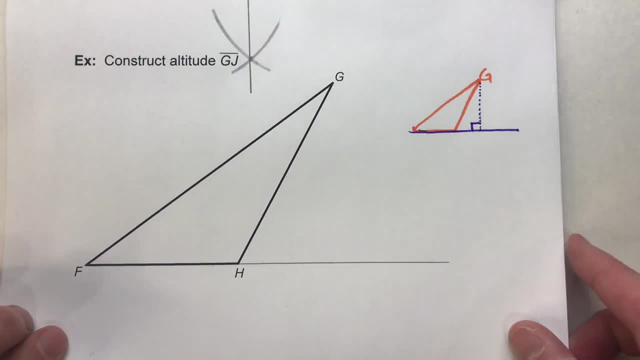 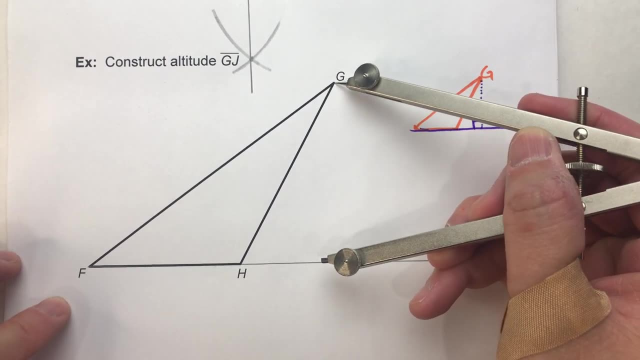 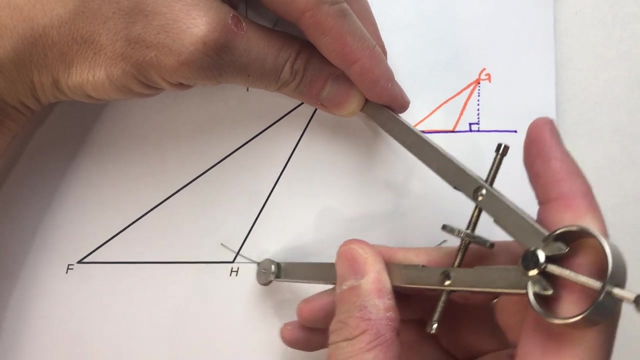 the way we did before. We're going to take our compass and we're going to set it. so it is big enough so that from point G I can hit that line in two places. need to be a little bit bigger. There we go, Swing an arc, hit that line in two places here and here And now. 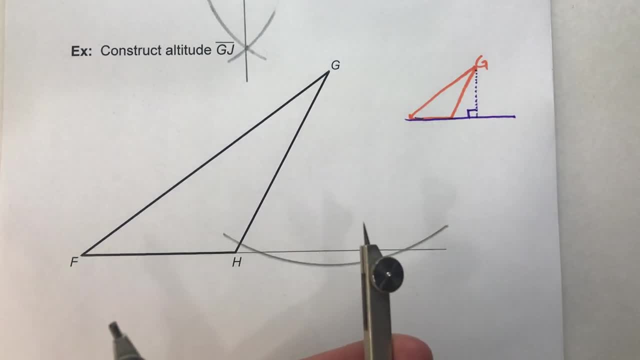 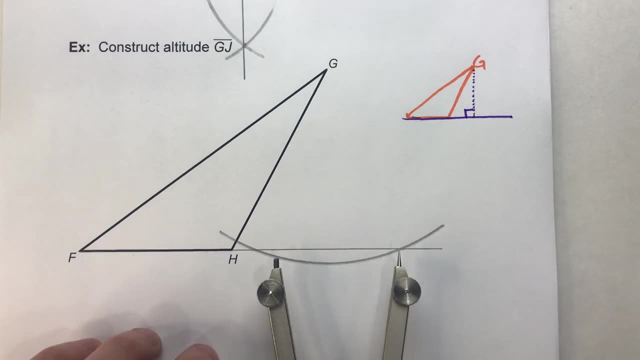 I'm going to change my compass setting So it's a little smaller, because I'm a little short in space here. Now we need to find another point to draw our altitude through. Okay, so compass setting more than half the distance from where the arcs hit the line.